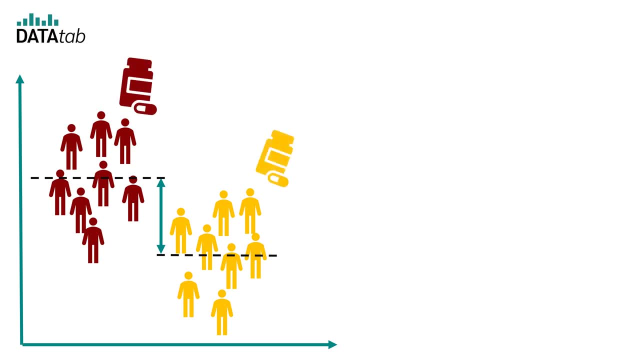 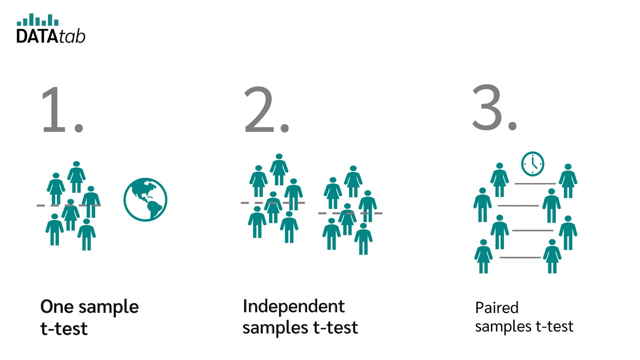 who received once drug A and once drug B. We would now like to know if there is a difference in blood pressure between these two groups. Now, there are three different types of t-tests: The one-sample t-test, the independent-samples t-test and the paired-samples t-test. 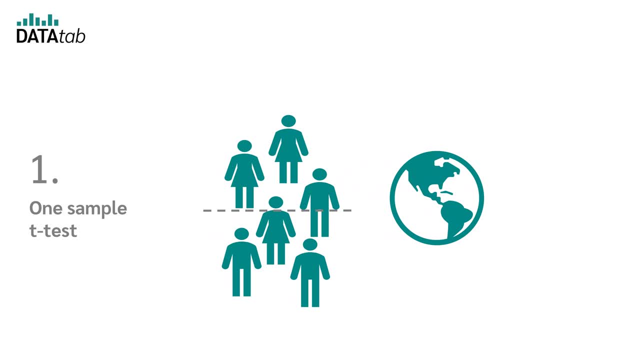 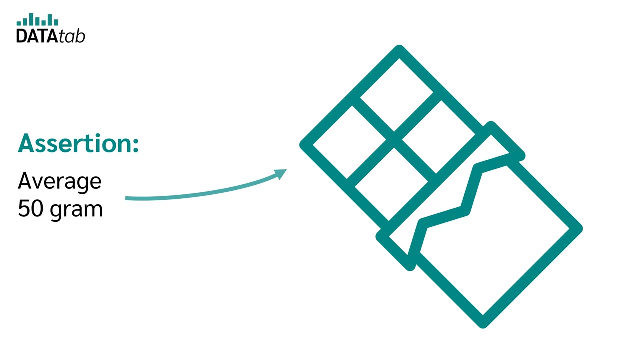 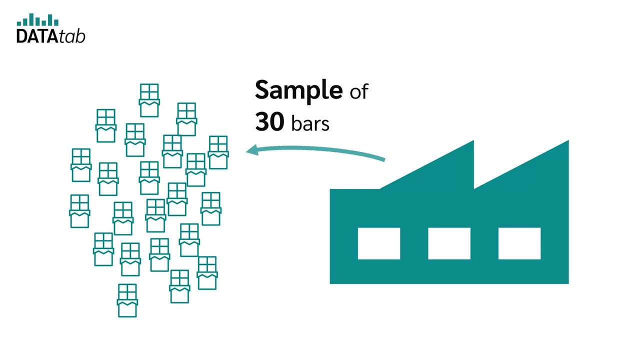 When do we use a one-sample t-test? We use the one-sample t-test when we want to compare the mean of a sample with a known reference mean. A chocolate bar manufacturer claims that its chocolate bars weigh an average of 50 grams. To check this, we take a sample of 30 bars and weigh them. The mean value of this sample. 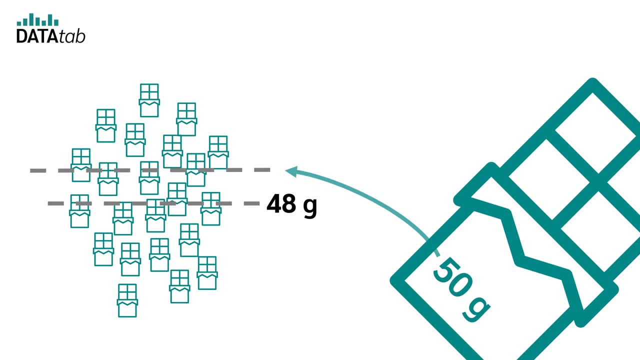 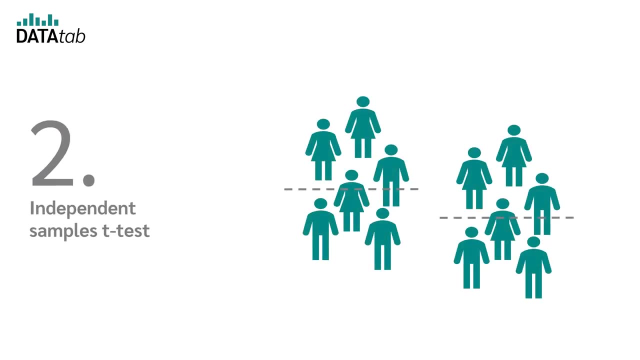 is 48 grams. Now we can use a one-sample t-test to check if the mean of 48 grams is significantly different from the claimed 50 grams. When do we use the independent-samples t-test? We use the t-test for independent samples. 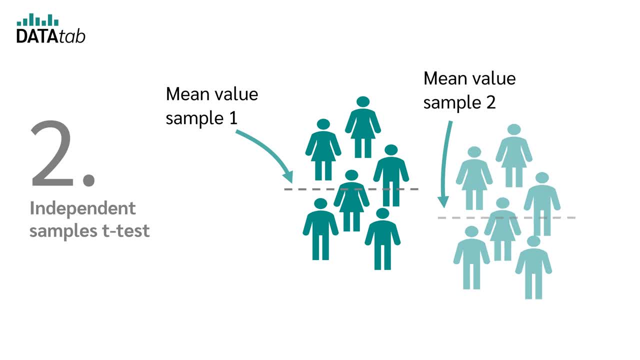 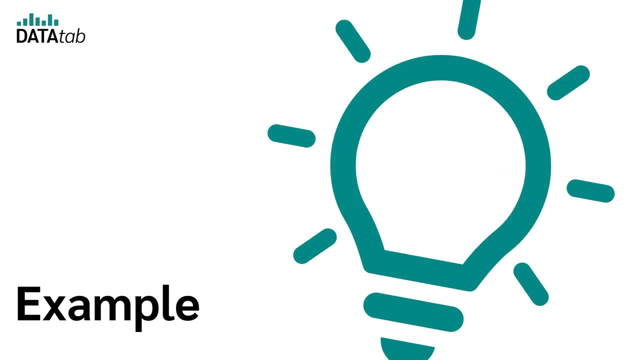 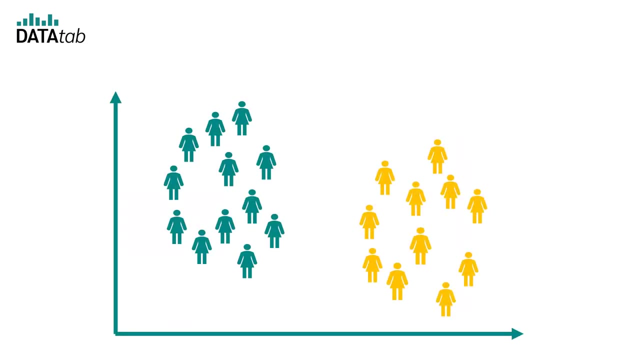 when we want to compare the means of two groups. We want to know if there is a significant difference between these means. we would like to compare the effectiveness of two painkillers. We randomly divide 60 people into two groups. The first group receives drug A and the second 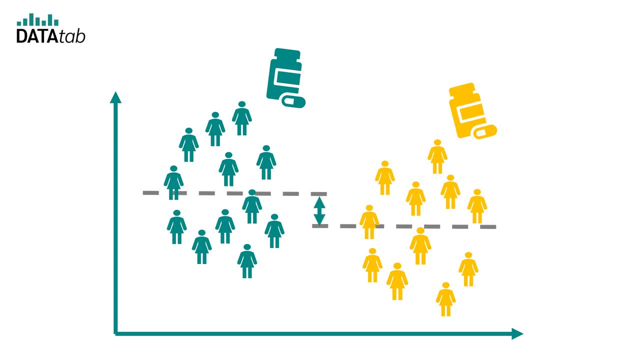 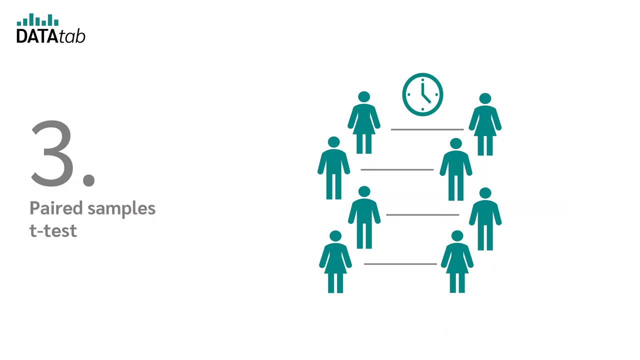 group receives drug B. Using an independent t-test, we can now test whether there is a significant difference in painkillers. We can now measure the pain relief between the two drugs When we use the paired-samples t-test. we use the paired-samples t-test to compare the 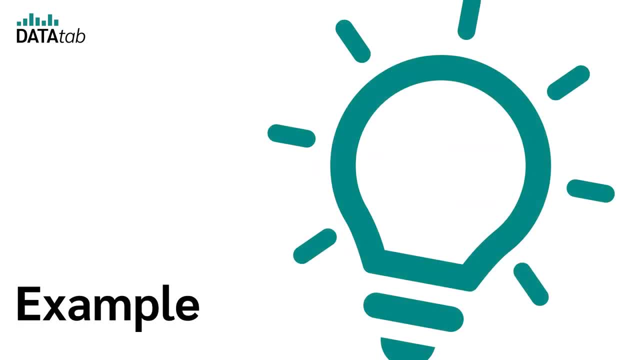 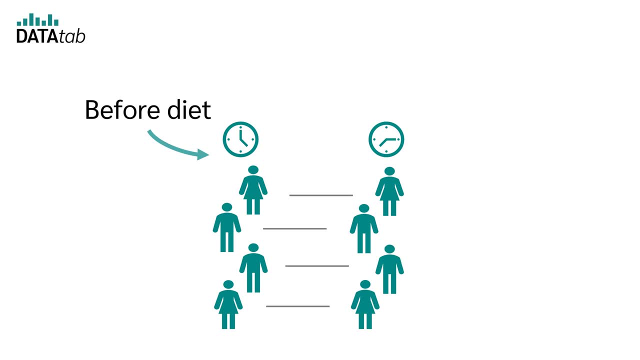 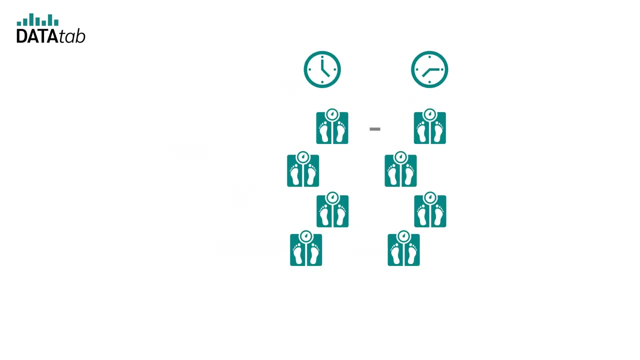 means of two dependent groups. we want to know how effective a diet is. To do this, we weigh 30 people before the diet and then weigh exactly the same people after the diet. Now we can look at the difference in weight between before and after the diet. 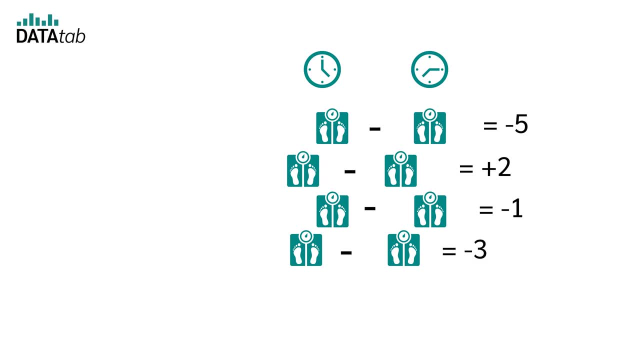 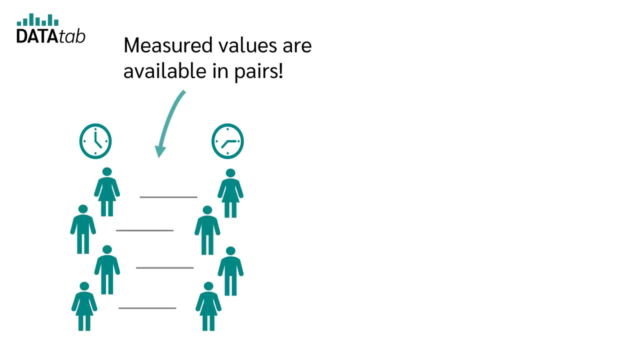 We can measure the weight of a person after the diet and then measure the weight of a and after for each subject. We can now use a paired samples t-test to test whether there is a significant difference In a paired sample. the measurements are available in pairs. The pairs result, for example, from repeated 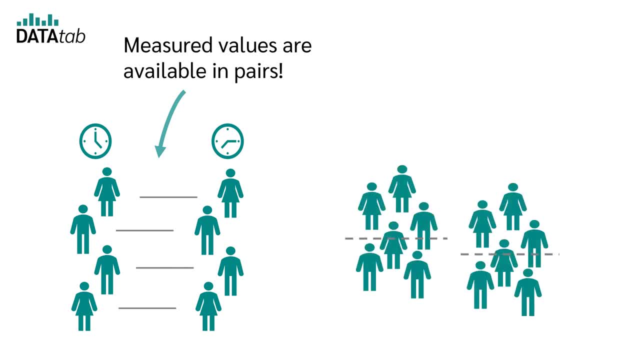 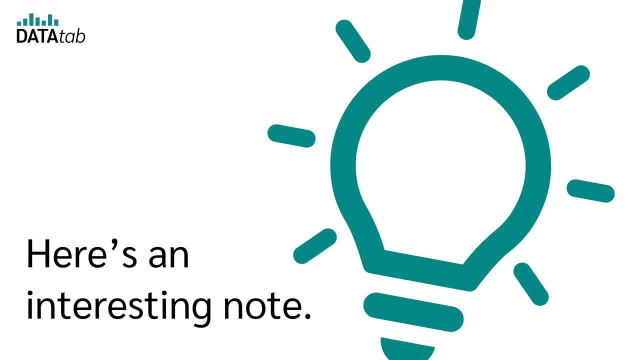 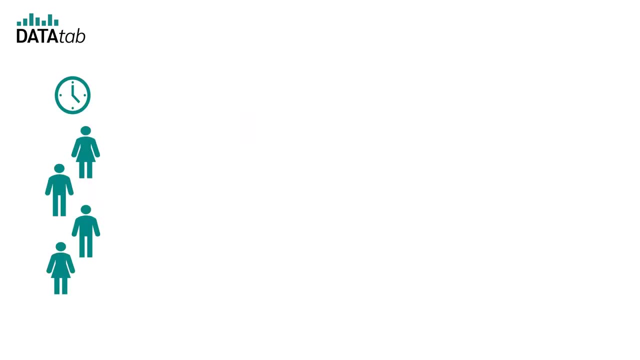 measurements with the same people. Independent samples are made up of people and measurements that are independent of each other. Here's an interesting note: The paired samples t-test is very similar to the one sample t-test. We can also think of the paired samples t-test as having one. 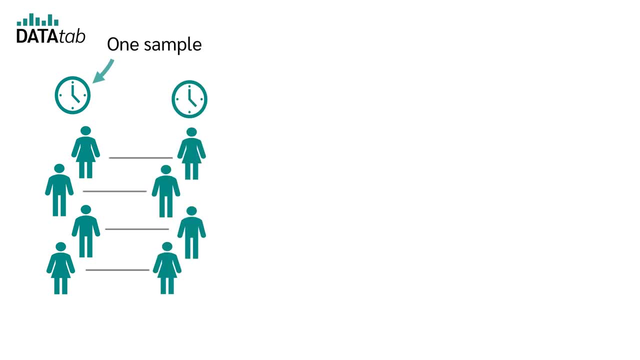 sample that was measured at two different times. We then calculate the difference between the paired values, giving us a value. for one sample. The difference is once minus five, once plus two, once minus one and so on and so on. Now we want to test whether the mean value of the difference just. 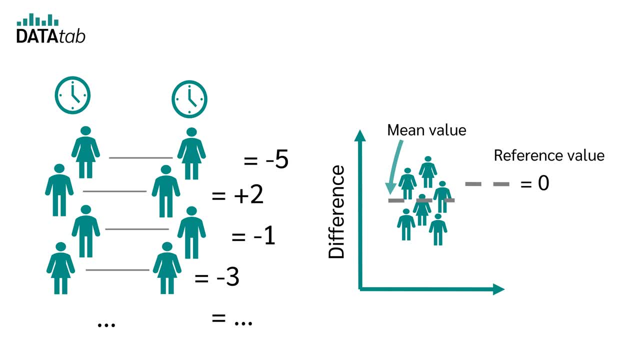 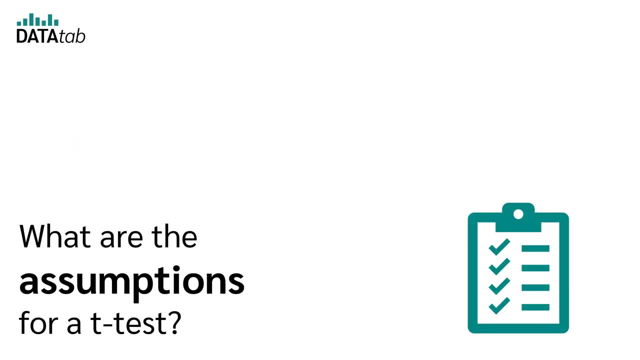 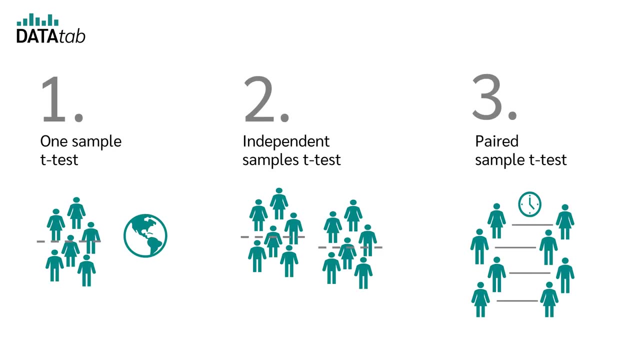 calculated deviates from a reference value, In this case zero. This is exactly what the one sample t-test does. What are the assumptions for a t-test? Of course, we first need a suitable sample In the one sample t-test. we need a sample and 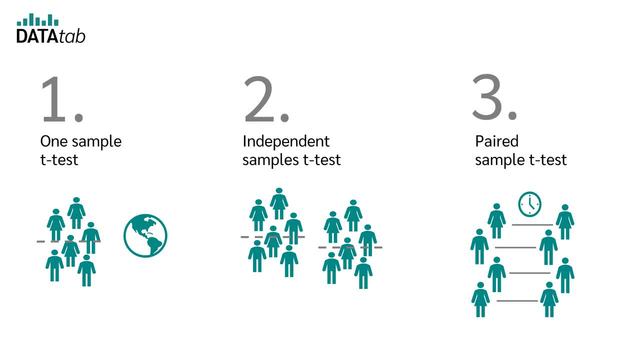 the reference value In the independent t-test, we need two independent samples And in the case of a paired t-test, a paired sample. The variable for which we want to test whether there is a difference between the means must be metric. Examples of metric variables are age, body weight and income, For example. 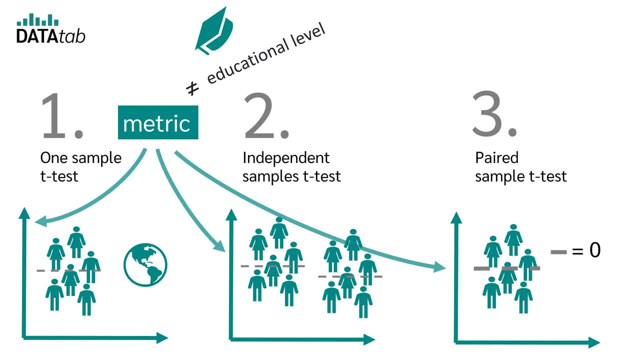 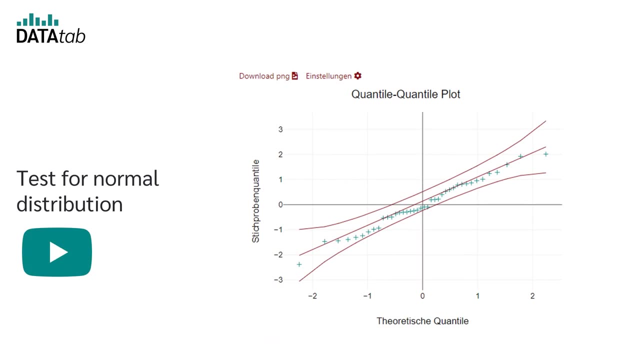 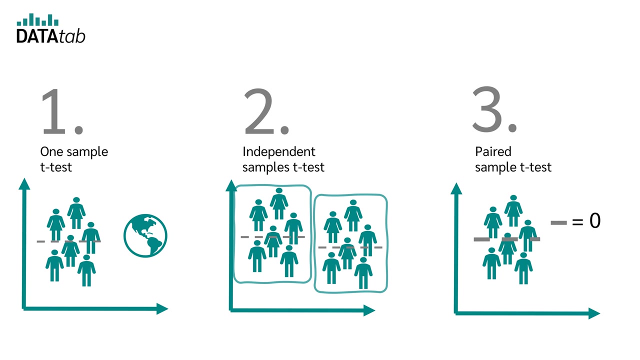 a person's level of education is not a metric variable. In addition, the metric variable must be normally distributed in all three t-test variants. To learn how to test if your data is normally distributed, watch my video. Tests for Normal Distribution. In case of an independent t-test, the variances in the two groups must be approximately equal. 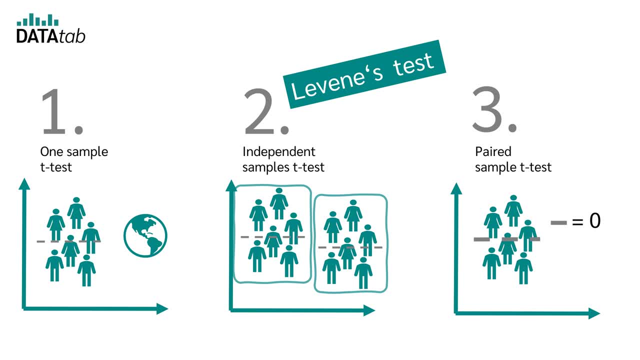 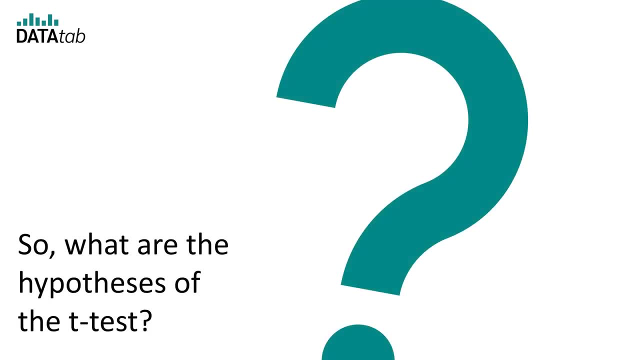 You can check whether the variances are equal using Levene's test. For more information, watch my video on Levene's test. So what are the hypotheses of the t-test? Let's start with the one sample t-test In the one. 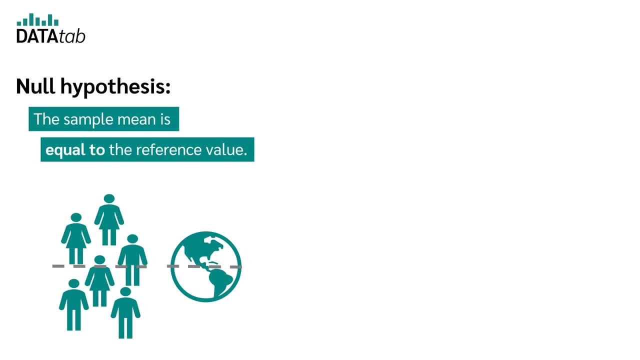 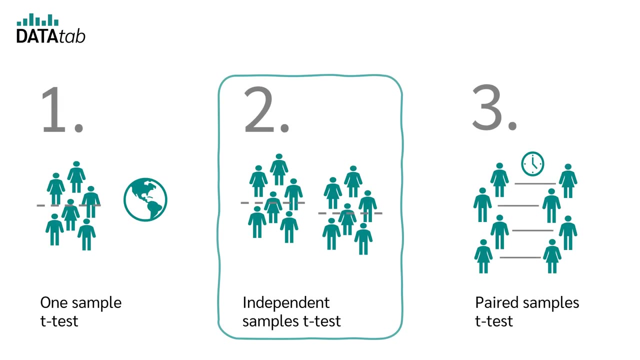 sample t-test. the null hypothesis is the sample mean is equal to the given reference value. So there is no difference. And the alternative hypothesis is the sample mean is not equal to the given reference value. What about the independent sample's t-test? 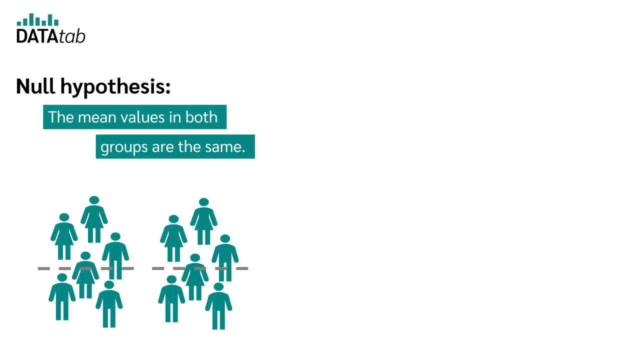 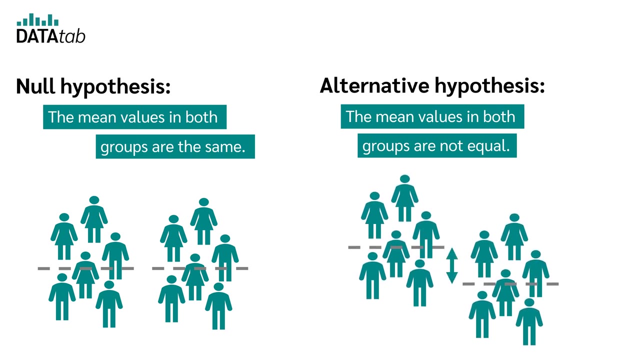 In the independent t-test, the null hypothesis is: the mean values in both groups are the same, So there is no difference between the two groups. And the alternative hypothesis is the mean values in both groups are not equal, So there is a difference between the two groups. 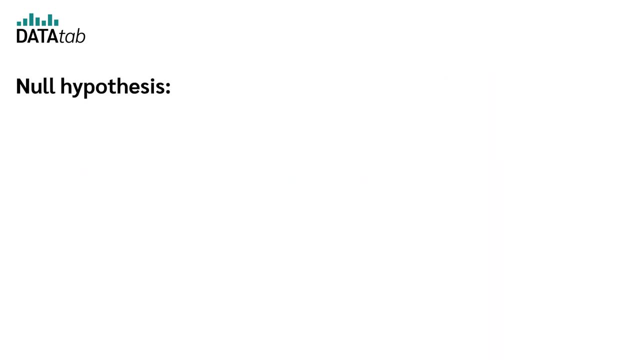 And finally the paired samples t-test. In a paired t-test, the null hypothesis is the mean of the difference between the pairs is zero, And the alternative hypothesis is the mean of the difference between the pairs is not zero. So now we know what the hypotheses are. 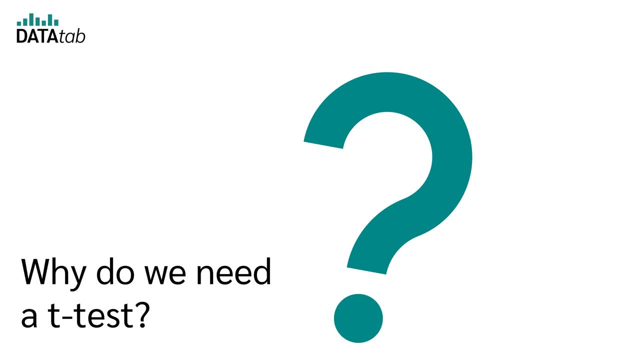 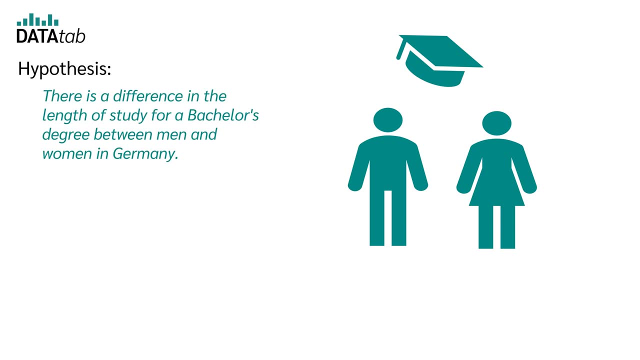 Before we look at how the t-test is calculated, let us look at an example of why we actually need a t-test. Let's say there is a difference in the length of study for a bachelor's degree between men and women. in Germany, Our population is 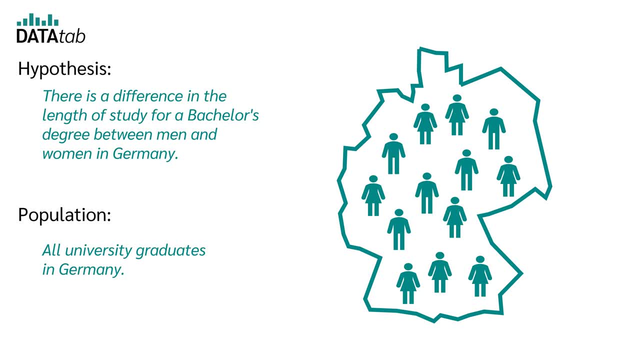 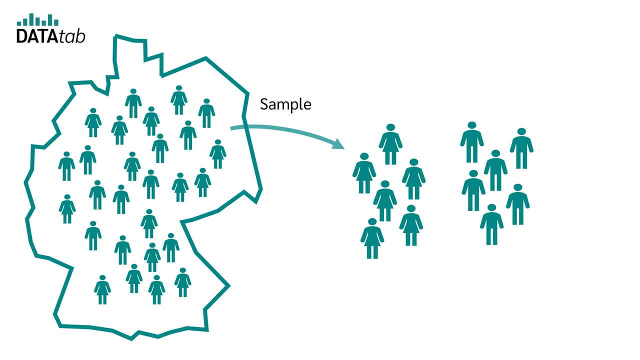 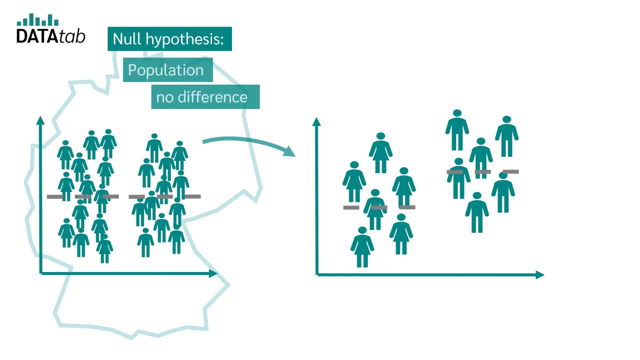 therefore made up of all graduates of a bachelor who have studied in Germany. However, as we cannot survey all bachelor graduates, we draw a sample that is as representative as possible. We now use the t-test to test the null hypothesis that there is no difference in the population. 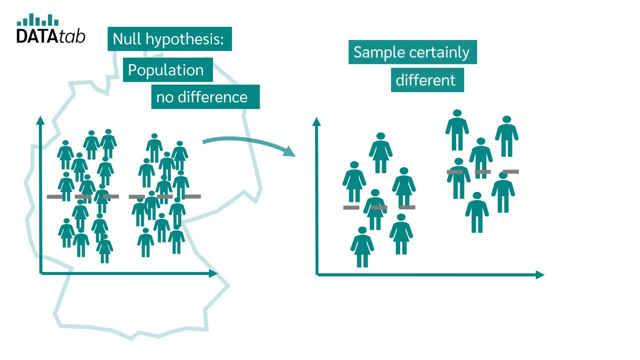 If there is no difference in the population, we will certainly still see a difference in study duration in the sample. It would be very unlikely that we drew a sample where the difference would be exactly zero. In simple terms, we now want to know at what difference, measured in a sample, we can say: 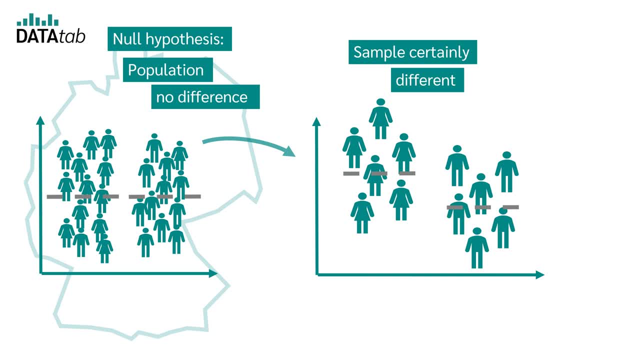 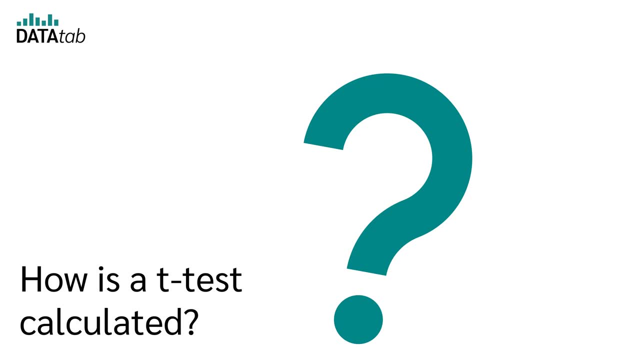 that the duration of the study is exactly zero. So we can say that the duration of the of study of men and women is significantly different, And this is exactly what the t-test answers. But how do we calculate a t-test? To do this, we first calculate the t-value. 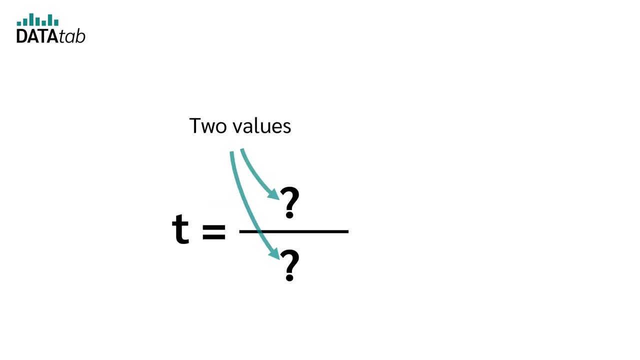 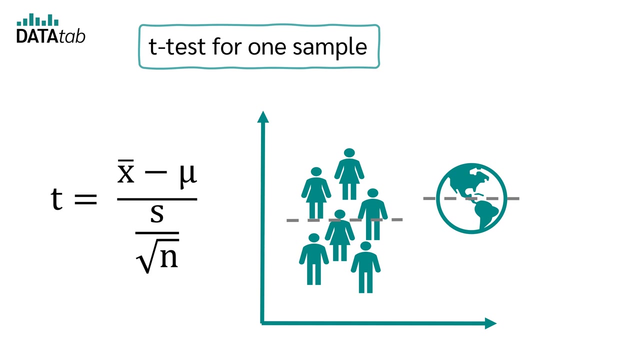 To calculate the t-value we need two values. First we need the difference between the means and then we need the standard deviation from the mean. This is also known as the standard error. In a one-sample t-test, we calculate the difference between the sample mean and the. 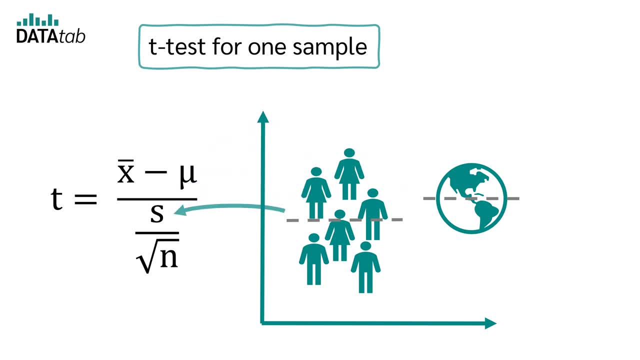 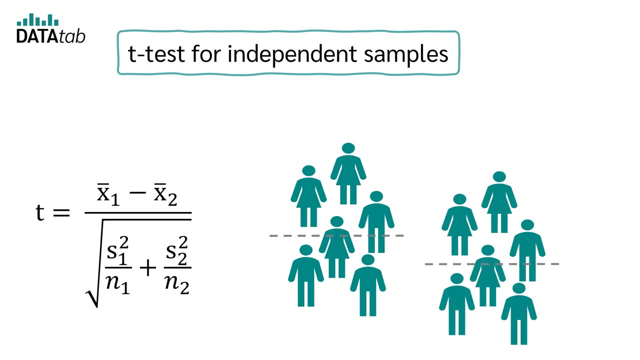 known reference mean. S is the standard deviation of the collected data and n is the number of cases. S divided by the square root of n is then the standard deviation from the mean, which is the standard error In a dependent samples- t-test. 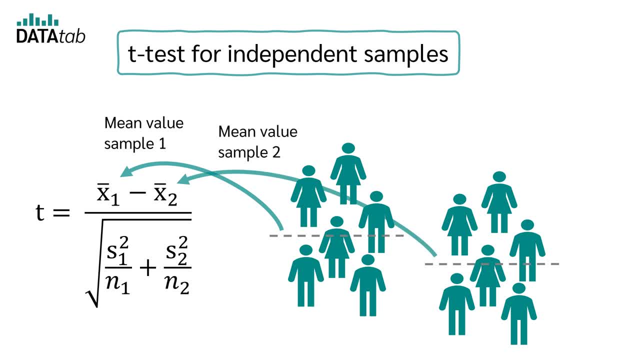 we simply calculate the difference between the two sample means. To calculate the standard error, we need the standard deviation and the number of cases from the first and second sample. Depending on whether we can assume equal or unequal variance for our data, there are different formulas for the standard error. Read more. 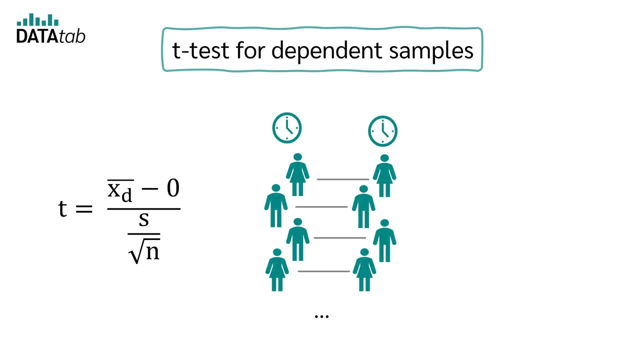 about this in our tutorial on datadepnet. In a paired sample t-test we only need to calculate the difference between the paired values and calculate the mean from that. The standard error is then the same as for a one-sample t-test. 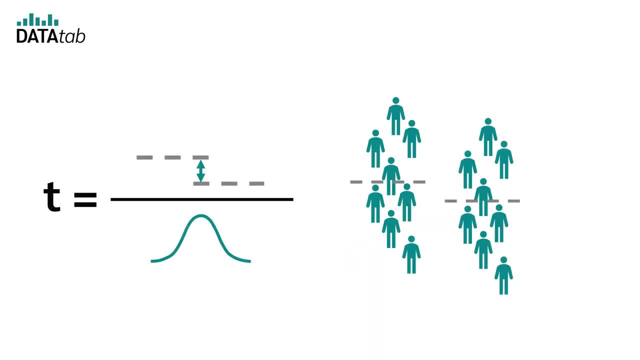 So what have we learned so far about the t-value? No matter which t-test we calculate, the t-value will be greater if we have a greater difference between the means, And the t-value will be smaller if the difference between the means is smaller. Further, the t-value becomes smaller when we have 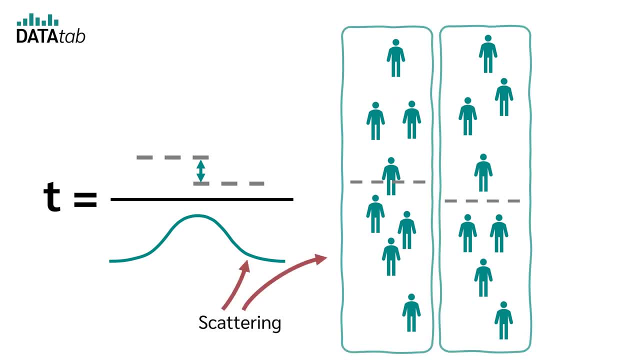 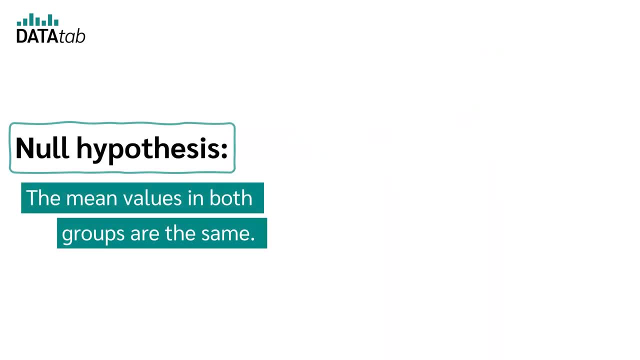 a larger dispersion of the mean. So the more scattered the data, the less meaningful a given mean difference is. Now we want to use the t-test to see if we can reject the null hypothesis or not. To do this, we can now use the t-value in two ways. Either we 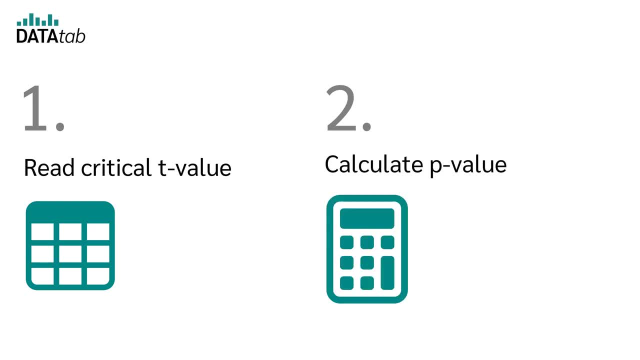 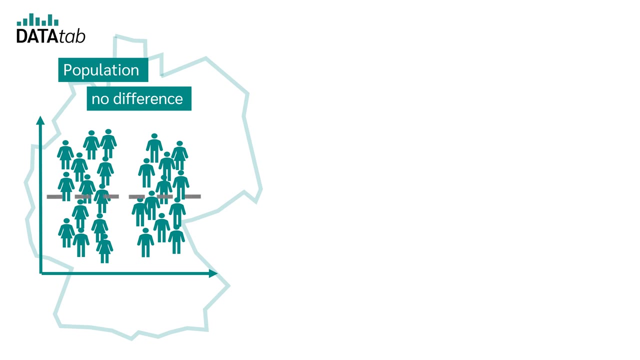 read the critical t-value from a table or we simply calculate the p-value from the t-value. We'll go through both in a moment. But what is the p-value? A t-test always tests the null hypothesis and the t-value, which shows us that there is no difference. So first we assume that there's. 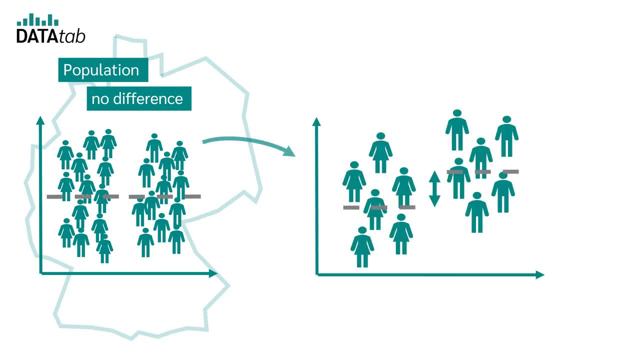 no difference in the population. When we draw a sample, this sample deviates from the null hypothesis by a certain amount. The p-value tells us how likely it is that we would draw a sample that deviates from the population by the same amount or more than a sample we drew Thus: 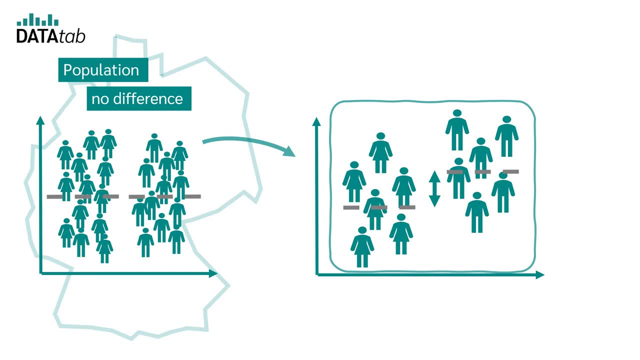 the more the sample deviates from the null hypothesis p-value becomes. If this probability is very, very small, we can of course ask whether the null hypothesis holds for the population. perhaps there is a difference, But at what point can we reject the null hypothesis? This border is called the significance level, which is usually 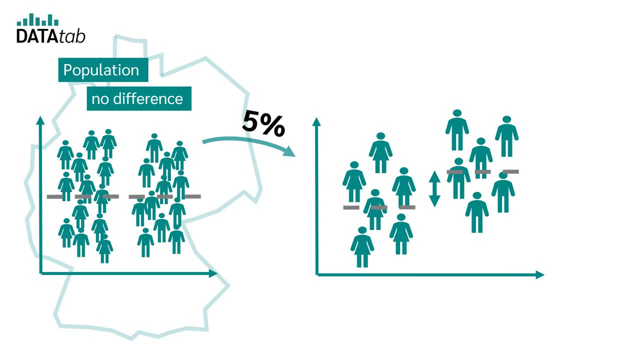 set at 5%. So if there is only a 5% chance that we draw such a sample or one that is more different, then we have enough evidence to assume that we reject the null hypothesis. And to put it simple, we assume that there is a difference, that the alternative hypothesis 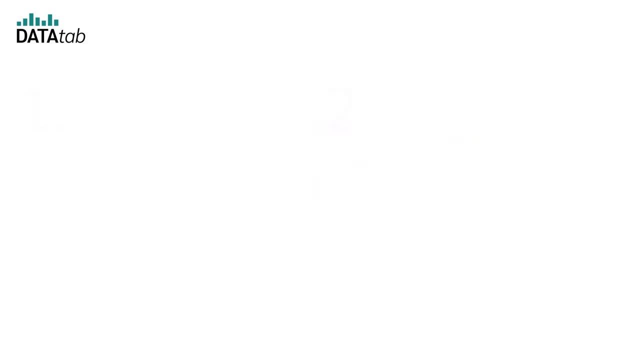 is true. Now that we know what the p-value is, we can finally look at how the t-value is used to determine whether or not the null hypothesis is rejected. Let's start with the path through the critical t-value, which you can read from a table To do. 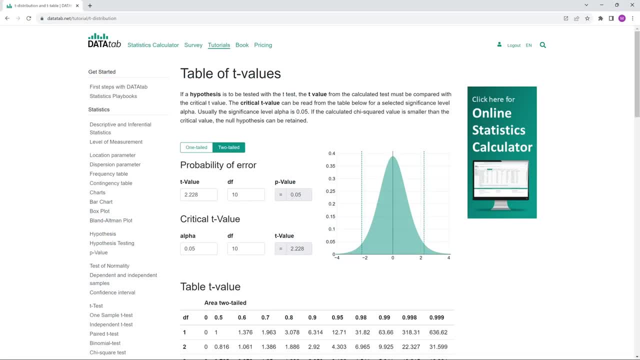 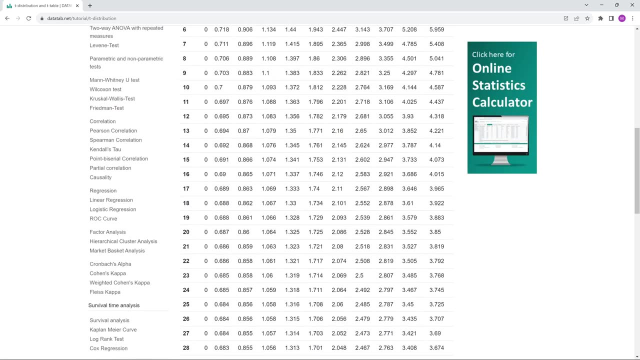 this click on the mouse button in the left corner э. We first need a table of critical t-values, which we can find on datadepnet under Tutorials and T-Distribution. Let's start with the two-tailed case. 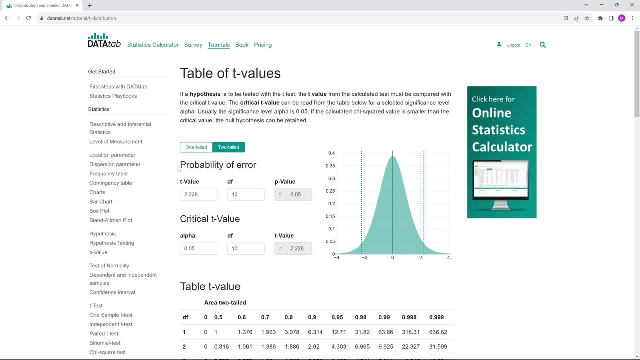 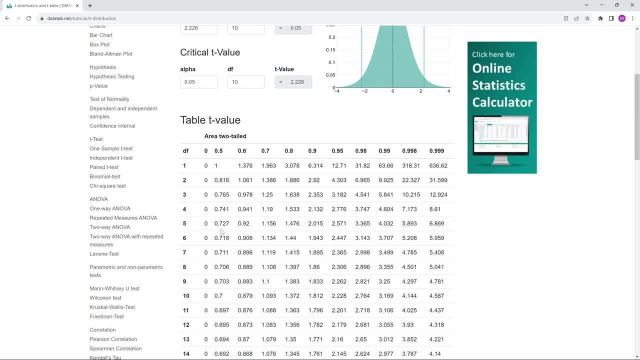 We'll briefly look at the one-tailed case at the end of this video. Here below we see the table. First, we need to decide what level of significance we want to use. Let's choose a significance level of 0.05 or 5%. 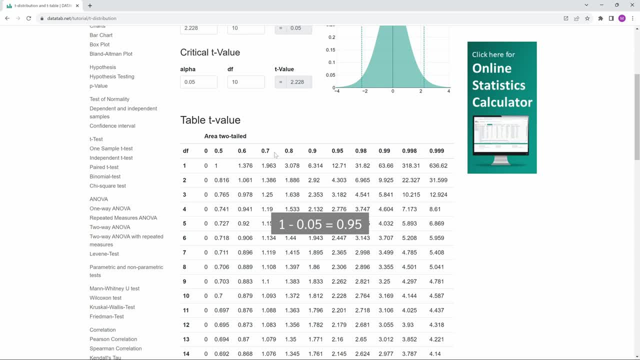 Then we look in this column at 1 minus 0.05, which is 0.95.. Now we need the degrees of freedom In the one-sample t-test and the paired-samples t-test. the degrees of freedom are simply the number of cases minus 1.. 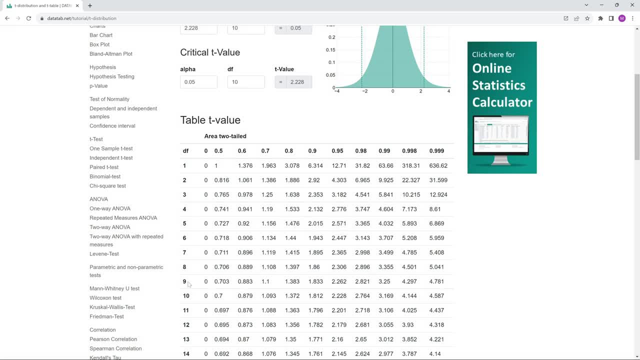 So if we have a sample of 10 people, there are 9 degrees of freedom In the independent-samples t-test. we add the number of people from both, We add the number of people from both samples and calculate that minus 2, because we have 2 samples. 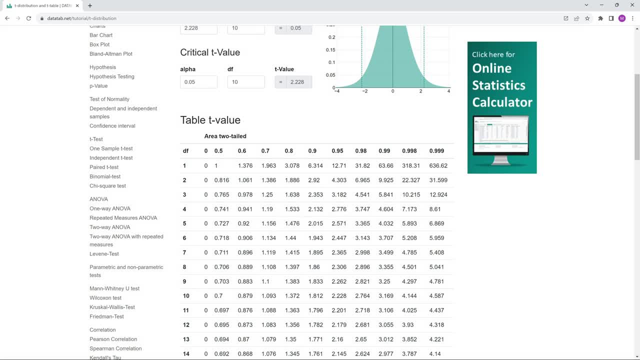 Note that the degrees of freedom can be determined in a different way depending on whether we assume equal or unequal variance. So if we have a 5% significance level and 9 degrees of freedom, we get a critical t-value of 2.262.. 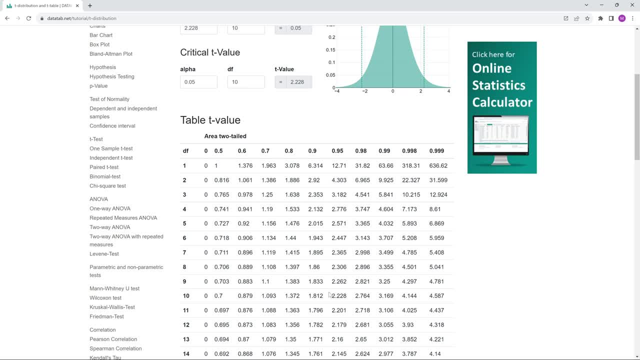 Now, on the one hand, we've calculated a t-value. with the t-value, We have the t-test and we have the critical t-value. If our calculated t-value is greater than the critical t-value, we reject the null hypothesis. For example, suppose we calculate a t-value of 2.5.. 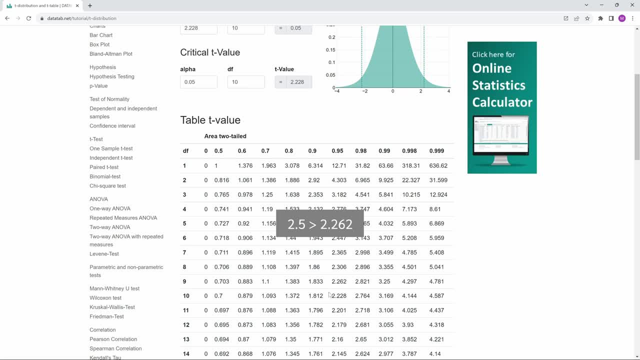 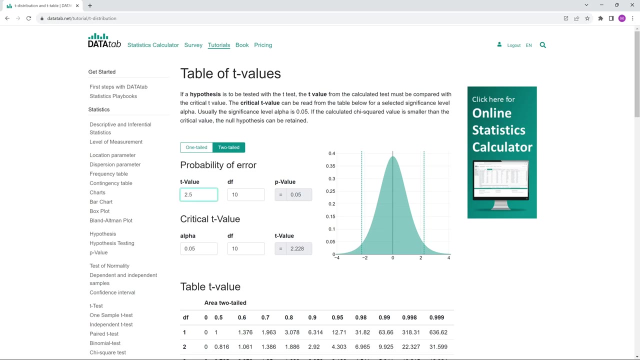 This value is greater than 2.262. And therefore the two means are so different that we can reject the null hypothesis. On the other hand, we can also calculate the p-value. If we enter 2.5 for the t-value and 9 for the degrees of freedom, we get a p-value of 0.034.. 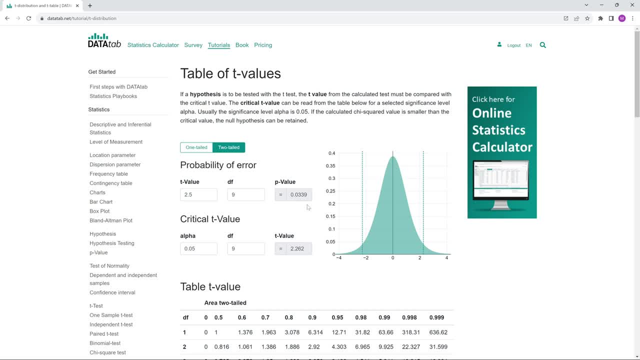 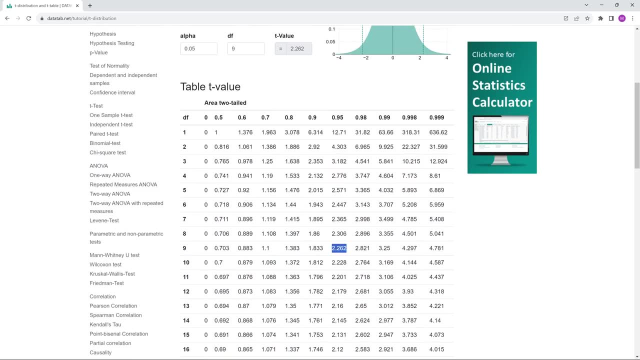 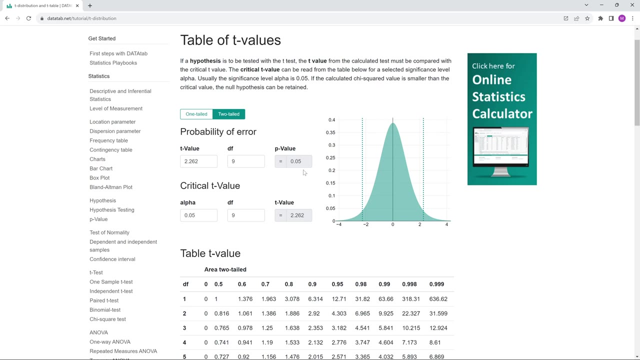 The p-value is less than 0.05 and we therefore reject the null hypothesis. As a control, we copy the t-value of 2.262. here We get exactly a p-value of 0.05.. Which is exactly the limit. 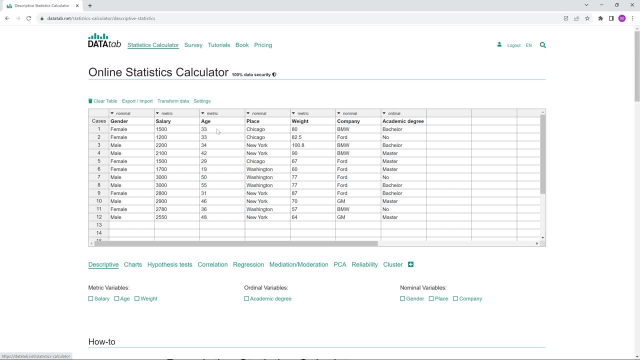 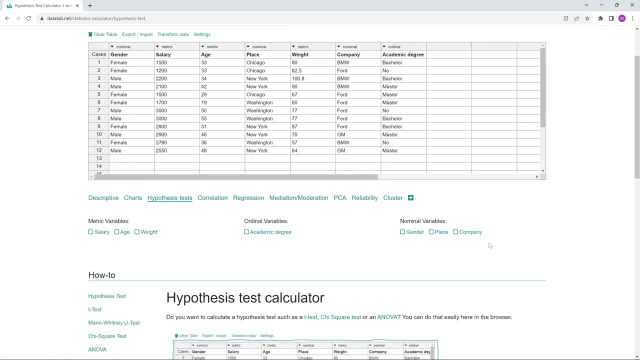 If you want to calculate a t-test with DataTab, you just need to copy your own data into this table, click on Hypothesis test and then select the variables of interest. For example, if you want to test whether gender has an effect on income, you simply click. 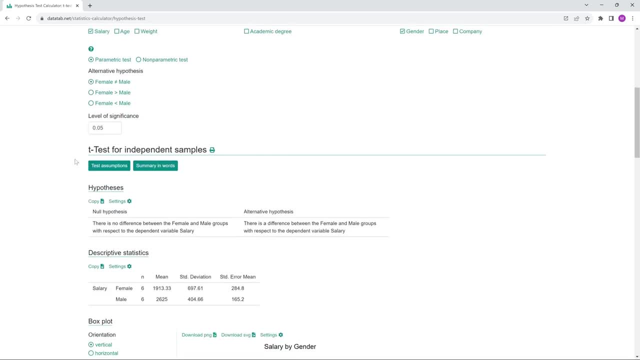 on the two variables and automatically get a t-test calculated for independent samples. Here below you can read the data. If you want to test whether gender has an effect on income, you simply click on the t-test and you can read the p-value. 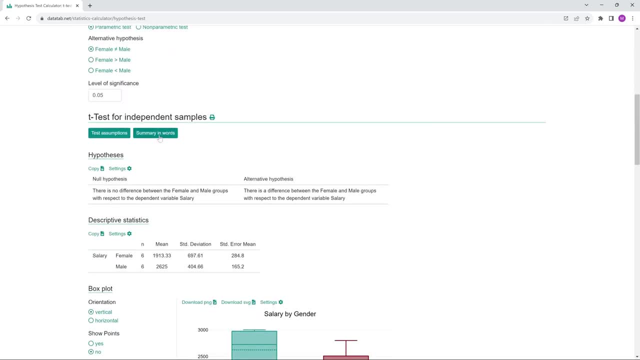 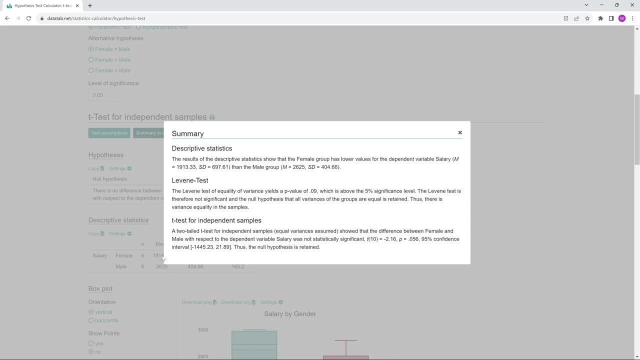 If you are still unsure about the interpretation of the results, you can simply click on Interpretation in Words. A two-tailed t-test for independent samples, equal variances assumed, showed that the difference between female and male with respect to the dependent variable salary was not statistically. 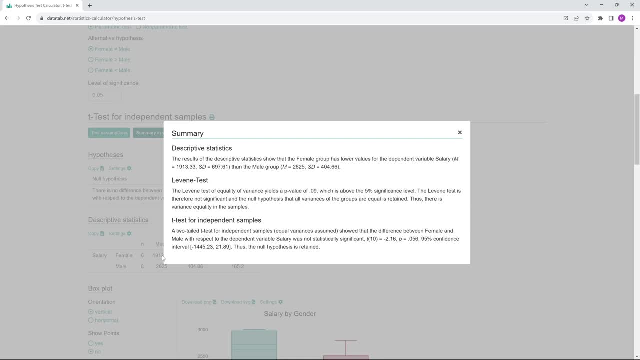 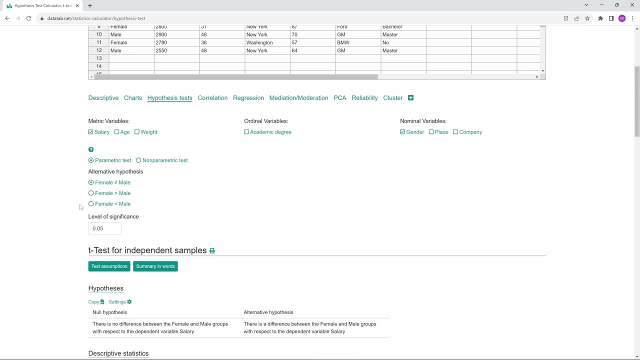 significant. Thus, the null hypothesis is retained. The final question now is: what is the difference between female and male with respect to the dependent variable salary? The final question now is: what is the difference between direct hypothesis and undirected hypothesis? In the undirected case, the alternative hypothesis is that there is a difference. 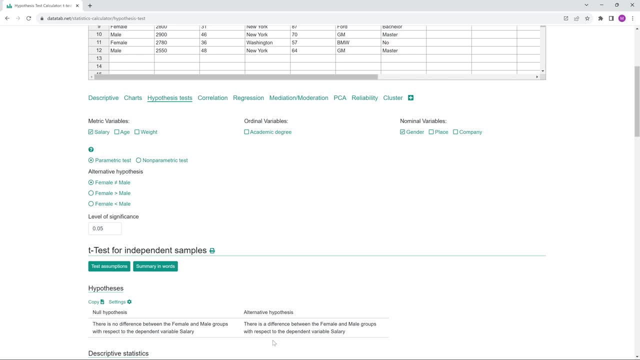 For example, there is a difference between the salary of men and women in Germany. We don't care who earns more, we just want to know if there is a difference or not. In a directed hypothesis, we are also interested in the direction of the difference. 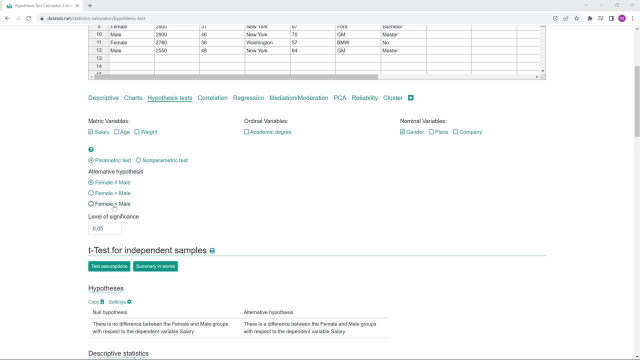 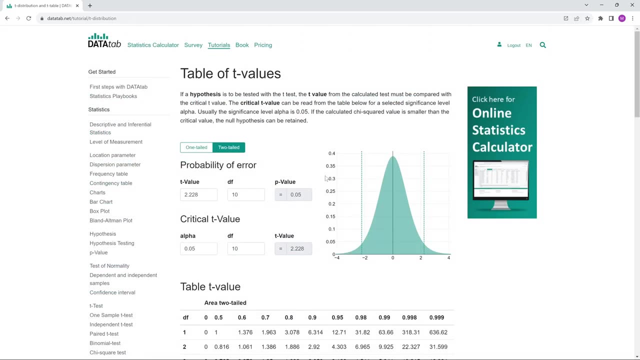 For example, the alternative hypothesis might be that men earn more than women or women earn more than men. If we look at the t-distribution graphically, we can see that in the two-sided case we have a range on the left and a range on the right. 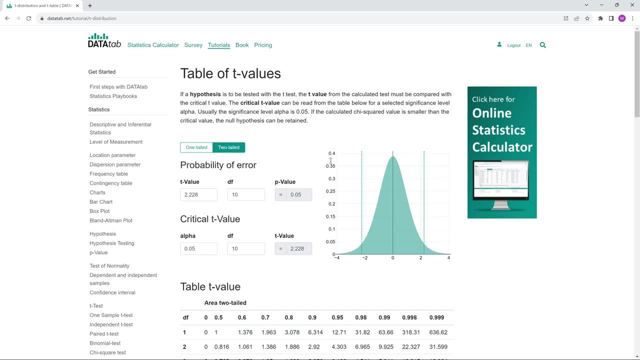 We want to reject the null hypothesis if we are either here or there With a 5% significance level, both ranges have a probability of 0.. If we do a one-tailed t-test, the null hypothesis is rejected only if we are in this range. 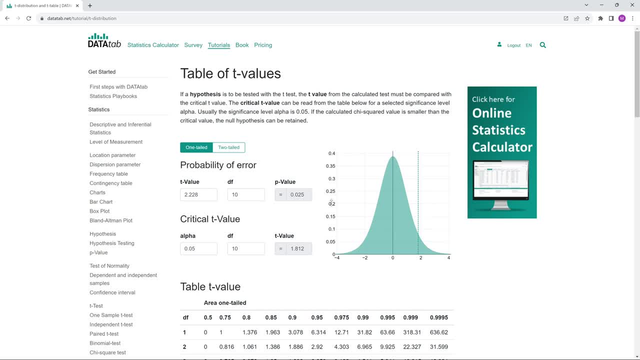 or depending on the direction which we want to test in that range, With a 5% significance level. all 5% fall within this range. I hope you enjoyed the video and see you next time. 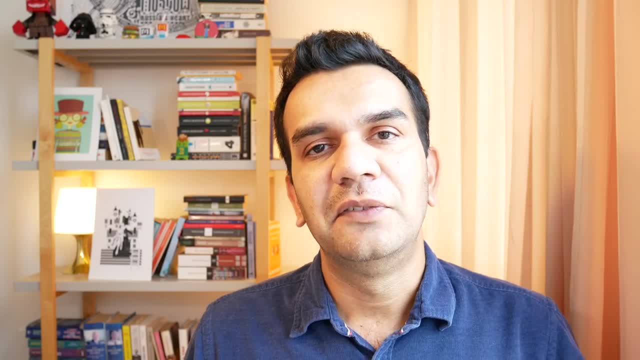 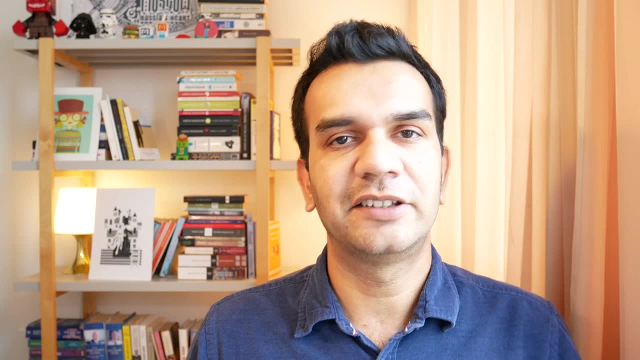 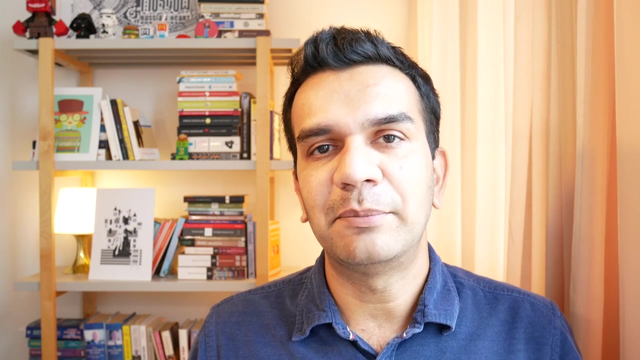 During the early days of the pandemic, we noticed that everyone was turning into some sort of an expert. People were dishing out advice as if they are statisticians or even doctors, And I don't have any such intention to talk about a field which I'm not aware. 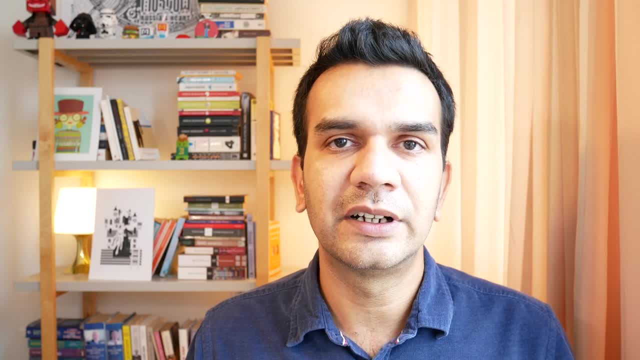 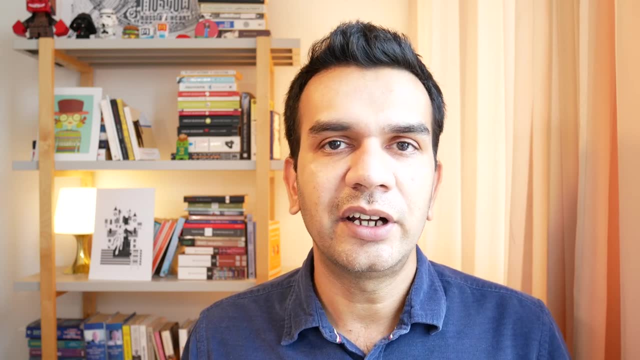 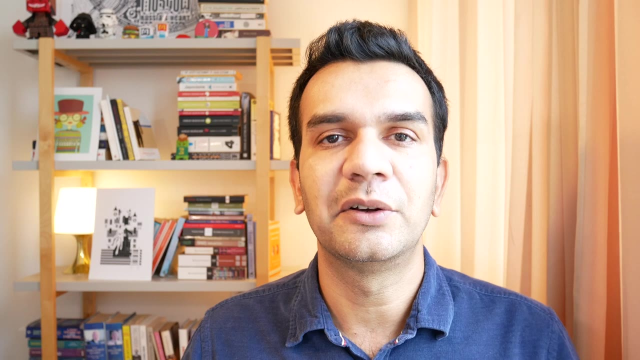 of. However, there is a term from the field of epidemiology which I found extremely interesting and it caught my attention, And that term is called R0.. R0 is basically the average number of people who will contract an infectious disease from a person who has that disease.